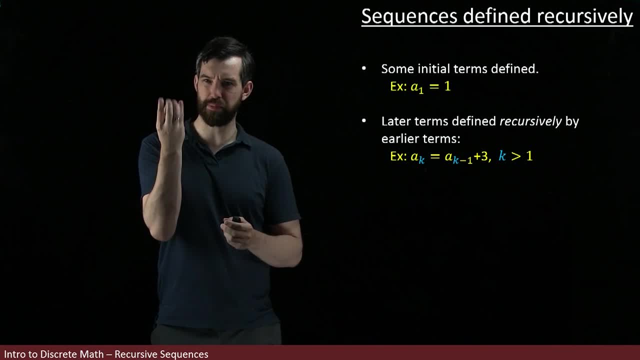 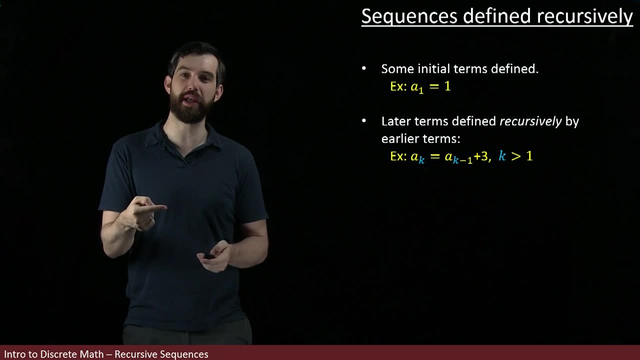 Now note that in this formula that the k is just a placeholder, I could put anything there. I could put some other symbol, I could put a box, I could also put some other relationship about k. So, for example, in this formula, what I've done is I've taken everywhere that there was a k up. 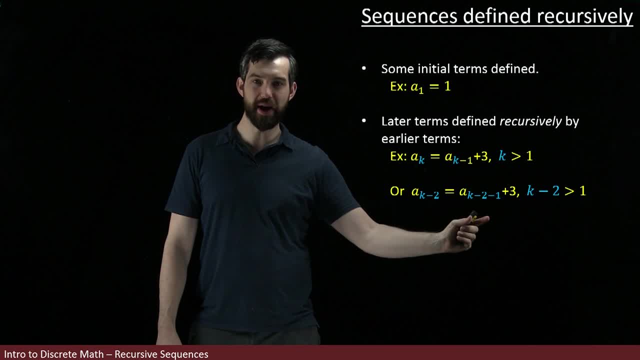 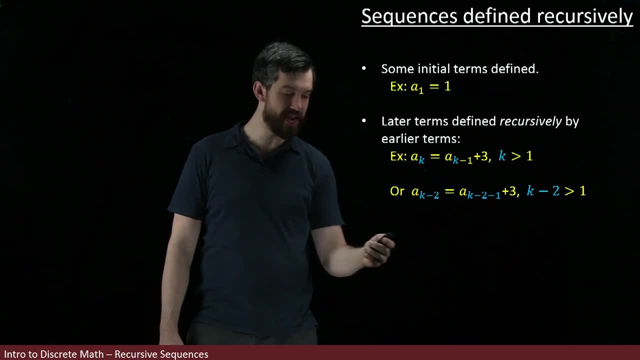 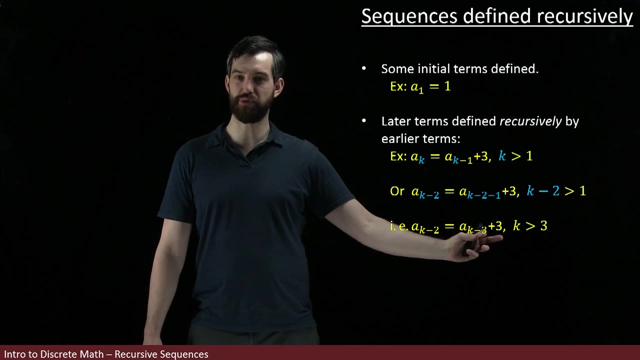 here and I've put in a k-2 here, a k-2 here and a k-2 there, And then maybe, if I go and do this algebra and I take the 2 to the other side, I can rewrite this as ak-2 is equal to ak-3 plus 3,. 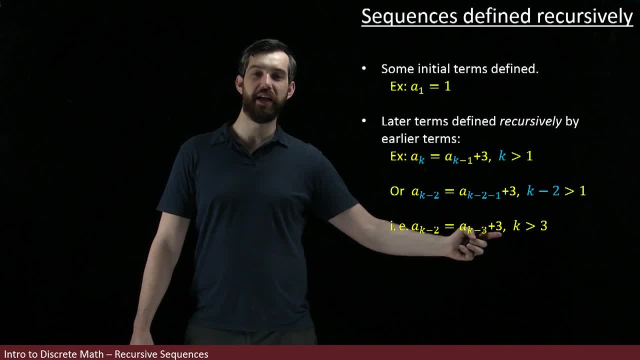 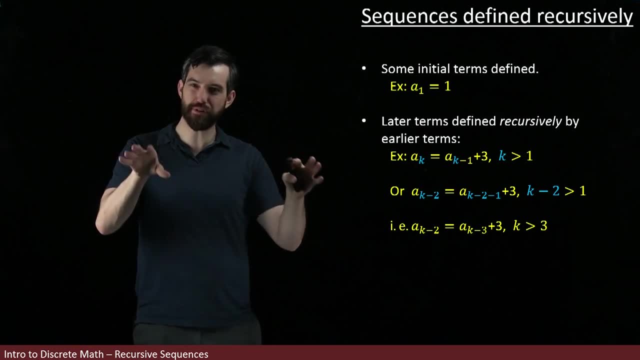 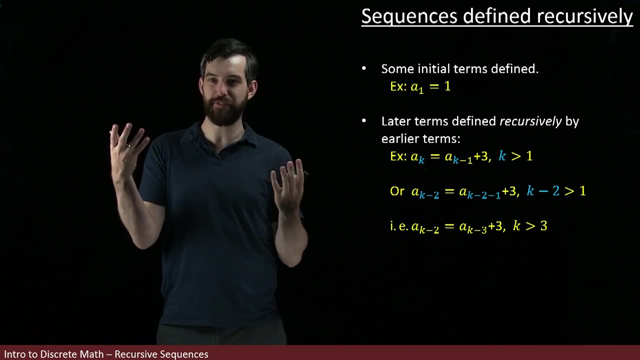 and that this formula is only valid in the space k being bigger than 3.. So the immediate takeaway is that these recursive formulas are not unique. The first one and this one that we've gone in down here are the same basic underlying sequence. 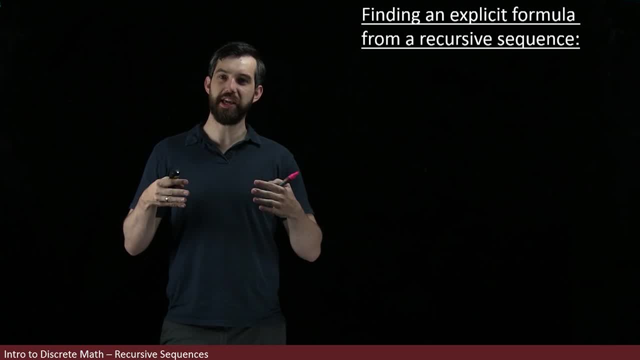 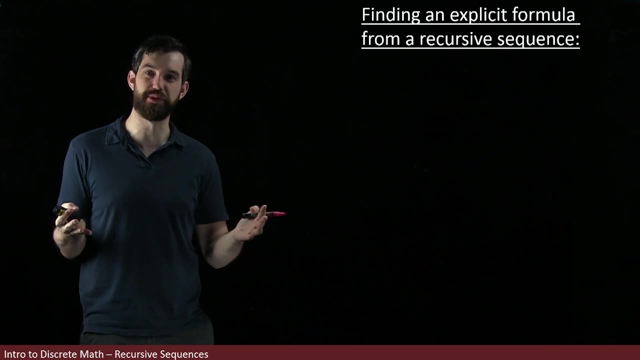 but they're just expressed in a bit of a different way. If a recursive formula is one that says the ak is defined in terms of previous ak's- ak-1,, ak-2, and so on- then an explicit formula is one that doesn't reference any other terms. 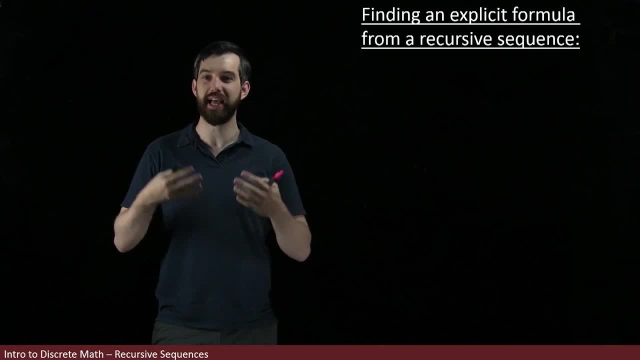 The only thing it references is that value k- It's ak- is some function. It's a function of k, like k-squared or k-factorial. So one of the goals that we have is: if I have a recursive sequence, can I find an explicit formula for it that is not recursive? 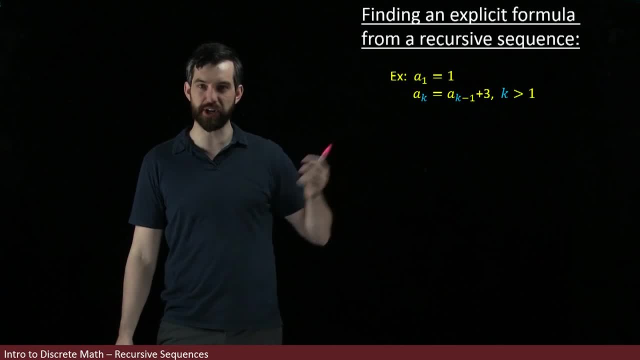 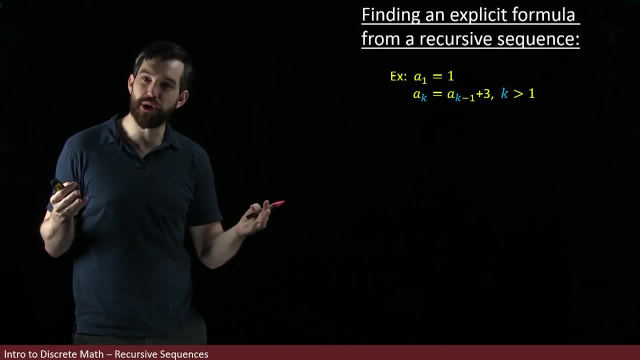 So let's look at the example that we had before. We've got this first term, the a1 is 1, and then the ak is given like this: I'm going to go and play around with this. I'm going to write out the first few terms. 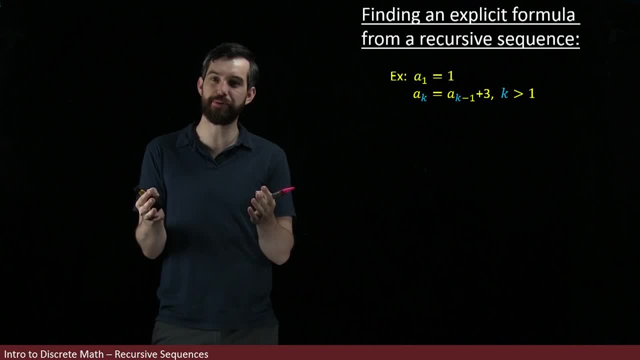 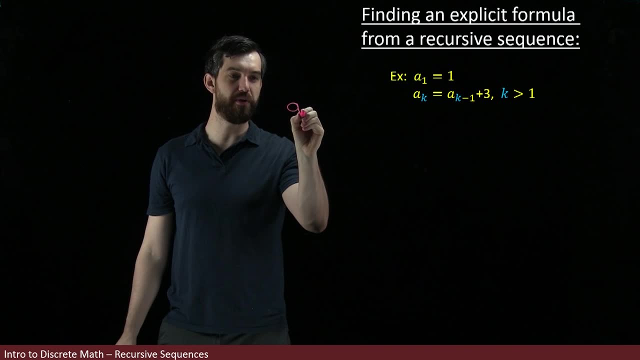 and I'm going to see if we notice some pattern and therefore we'll have an ability to write ak as a function only. So the a1 we know that's just given to us. We don't have to do any new work. 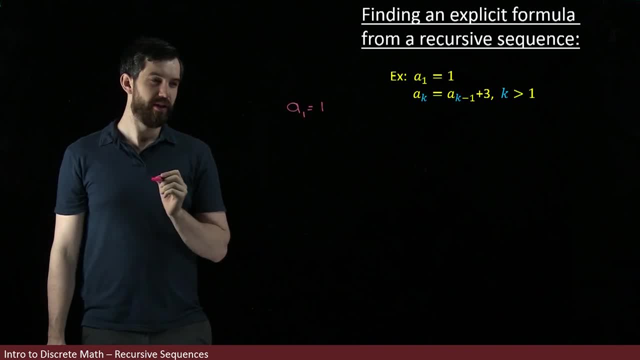 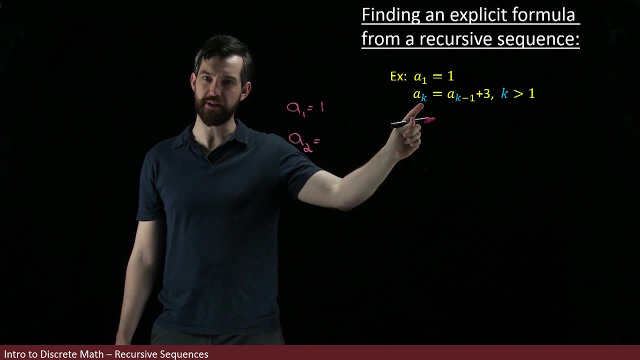 a1 is equal to 1.. Now let's do a2.. So what our formula tells us is that if I'm going to use k equal to 2 here, so this is a2, it's going to be whatever the value of a2 minus 1.. 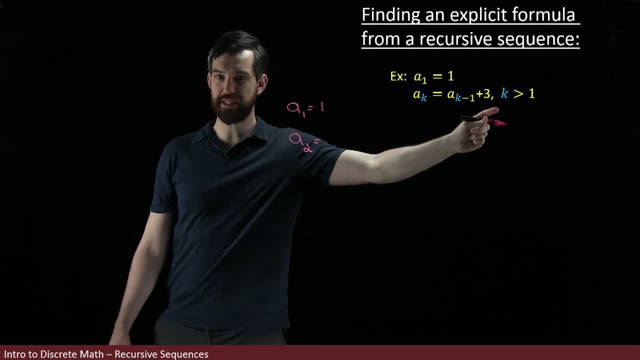 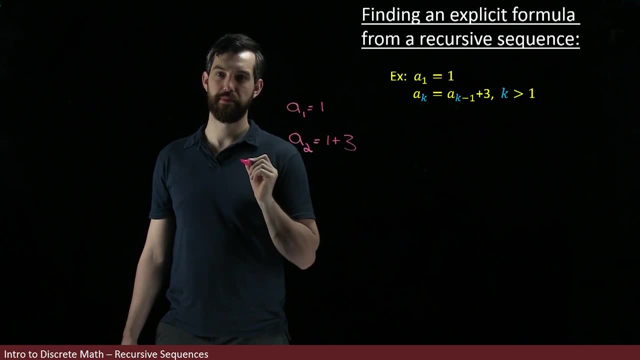 So a1 is plus 3.. So it's the a1 value, which was going to be a 1, and then I'm going to add to it 3.. And there I get my a1.. So I'm going to add to it 3.. 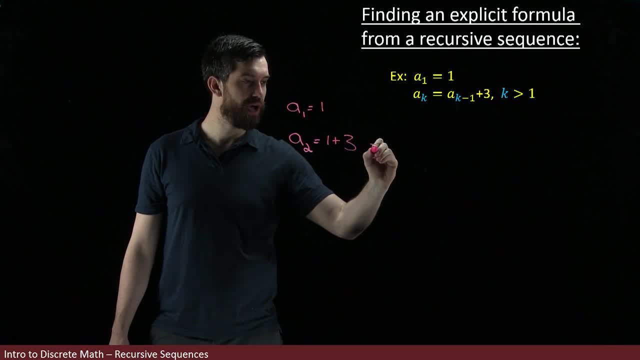 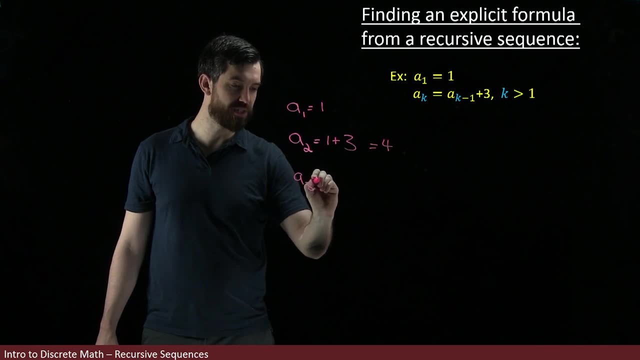 And there I get my a2, which we could then compute and was going to be equal to the value of 4.. So the first term is 1, the second term is 4.. Let's continue. If I look at what a3 is going to be, 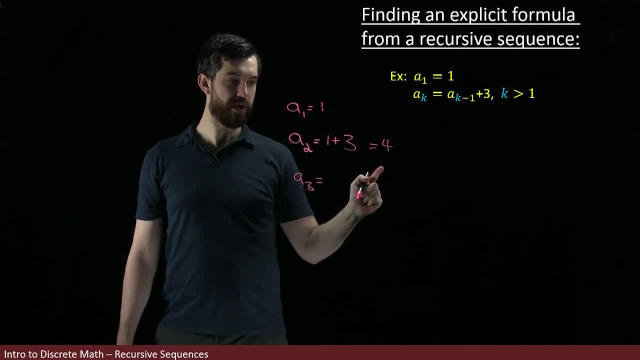 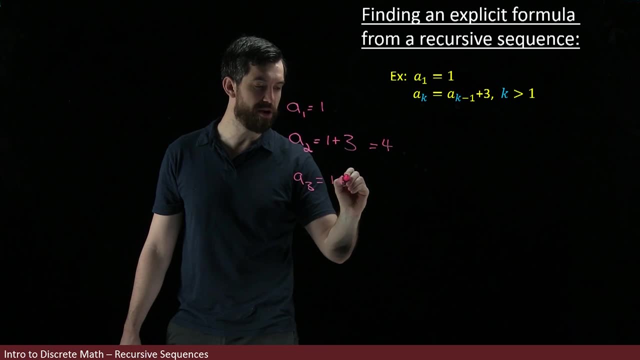 well, a3 is a2 plus 3.. So it's going to be 4 plus 3, but I'm actually going to keep it in its original format. I'm going to say that it's the a2, which I'll leave as the 1 plus the 3,. 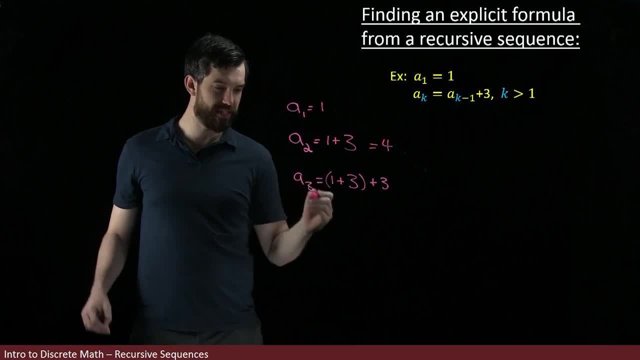 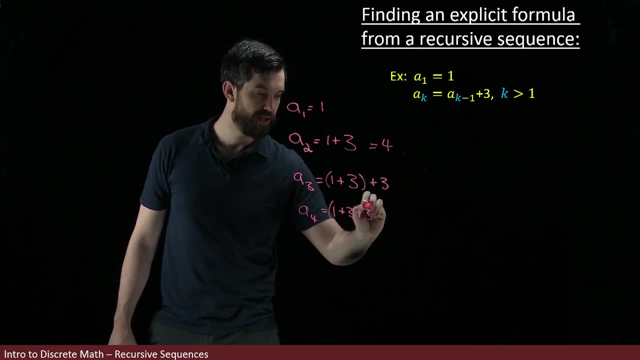 and then I'm going to add one more copy of 3.. Let's continue again. I'm now going to say that the a4 is equal to the 1 plus 3 plus 3.. So that was the value of my a3. 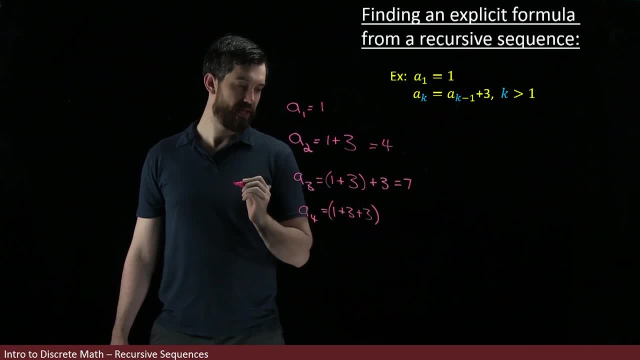 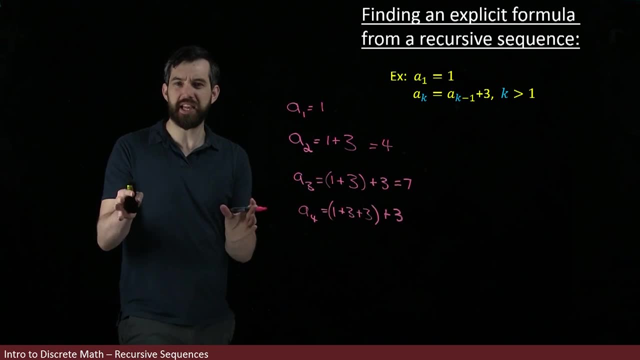 And this, of course, is just the same thing as 7,, but I'm not going to worry about that- And then we're going to add one more copy of 3.. So what it looks like is occurring here is that, because of this plus 3 that I have in my recursive formula, 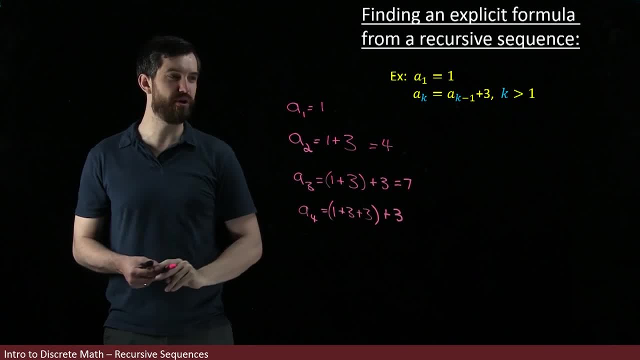 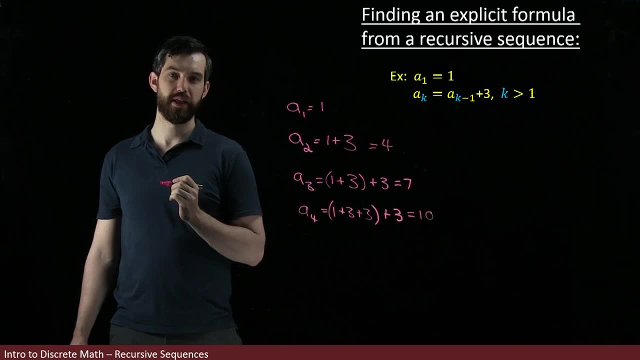 every time I go and do one of these terms, I'm adding 3 to it. 1 plus 3 is 4.. 4 plus 3 is 7.. 7 plus 3 is going to be equal to 10.. 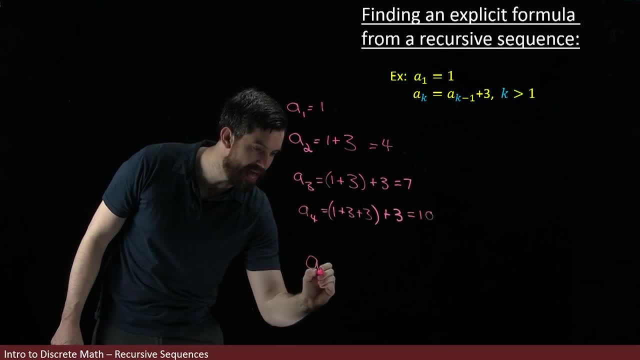 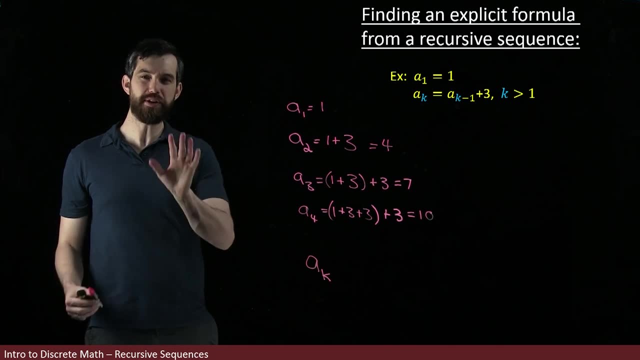 So now what I want to do is I want to write down my a, sub k, I want to write down the kth term to this sequence, And I want you to note the following fact: For a1, there were zero 3s. 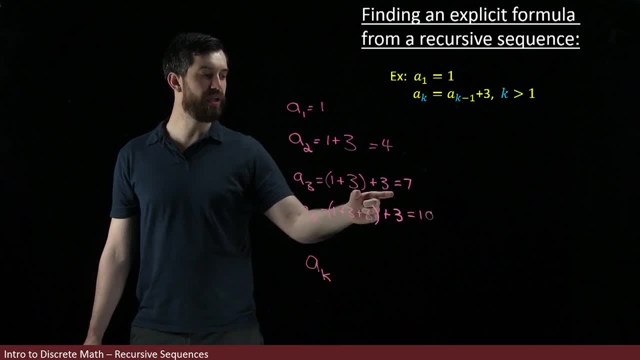 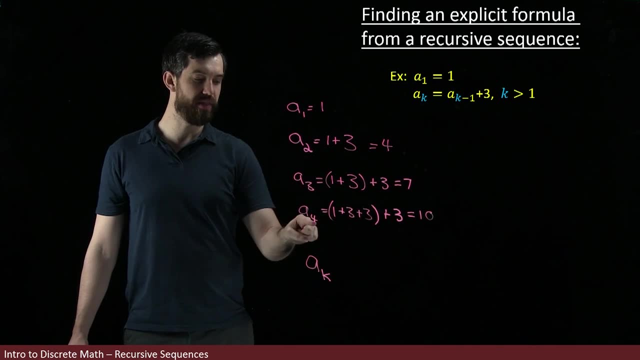 For a2, there was one: 3.. For a3, there was two 3s. For a4, there was three 3s. Notice how there's always one less 3 than the number that appears here, Like when the number is 4,. we're going to have three 3s. 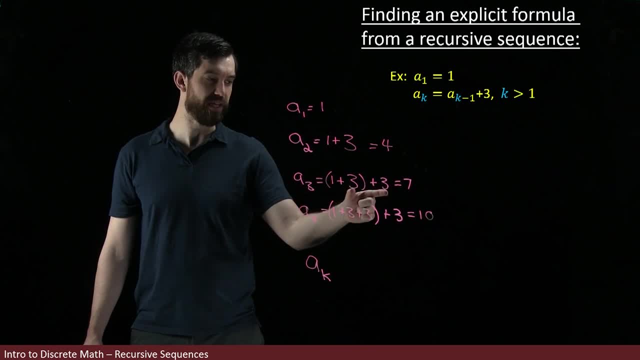 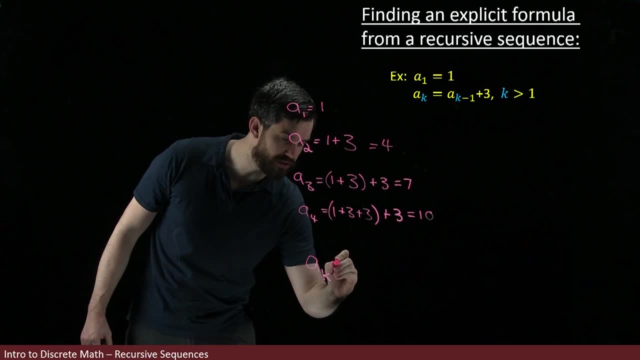 which is one less than 4.. When the number is 3,, we have two 3s, which is one less than 3.. So I believe that that's going to be the pattern. Every one of these terms is going to have the 1,. 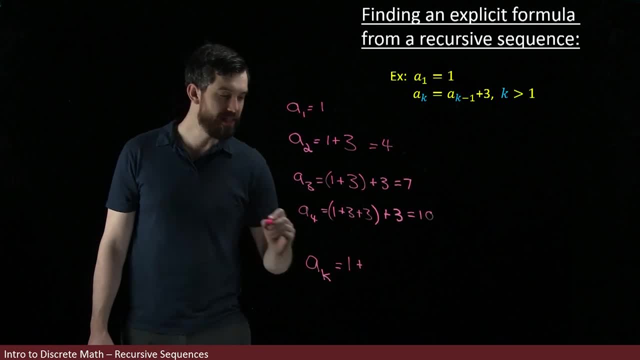 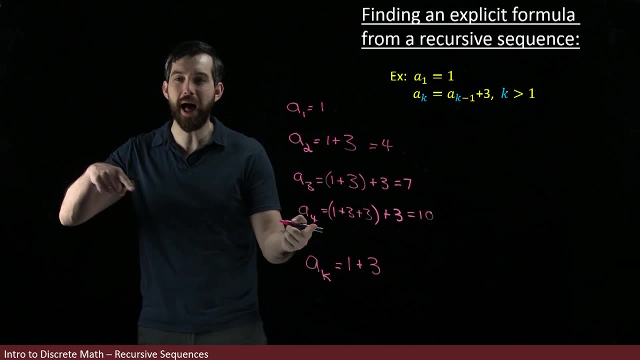 so the a k is definitely going to have a 1 out the front of it, And then it's got some number of 3s, but the number of 3s is the value k minus 1.. So I'm going to write it as 3k minus 1.. 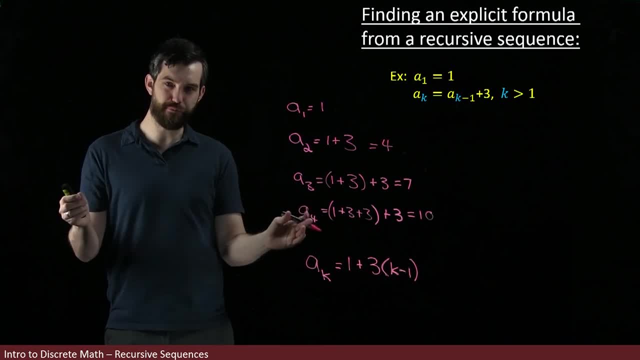 So this formula is the explicit formula for a k that comes about from this recursive definition for a k. Now, I believe we've done this accurately, but perhaps we've made a mistake. What I'm going to show you now is a verification. 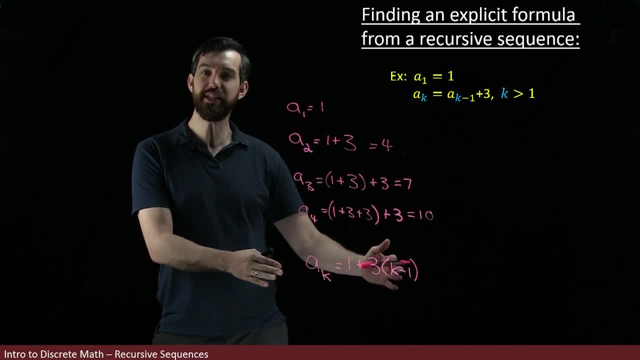 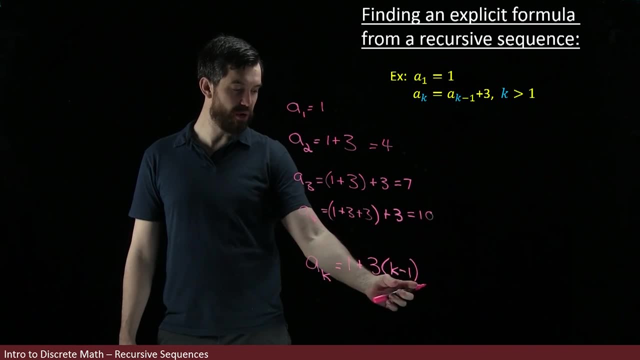 that the result that we have down here does indeed match this particular recursive formula. Clearly, in the case of k equal to 1, if I plug in k equal to 1, this is going to give me a 0. So for k equal to 1, it does indeed match. 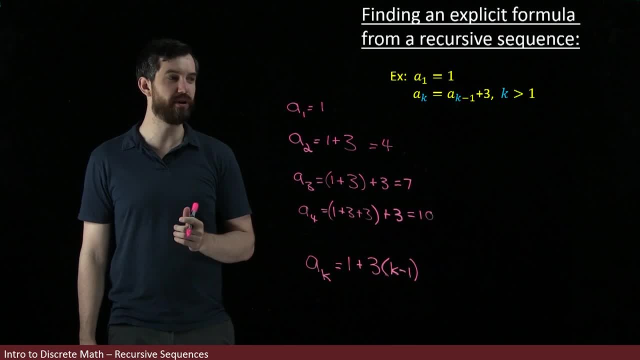 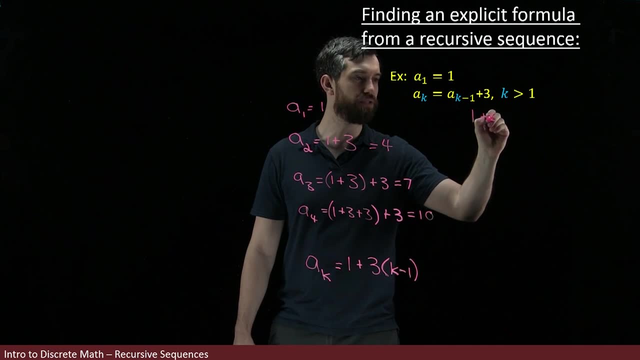 that my a 1 is equal to 1.. So that part's good, but it's the recursive part that I'm really interested in. So what I'm going to do here is I'm going to say that a k, which I just said was 1 plus 3 times k minus 1,. 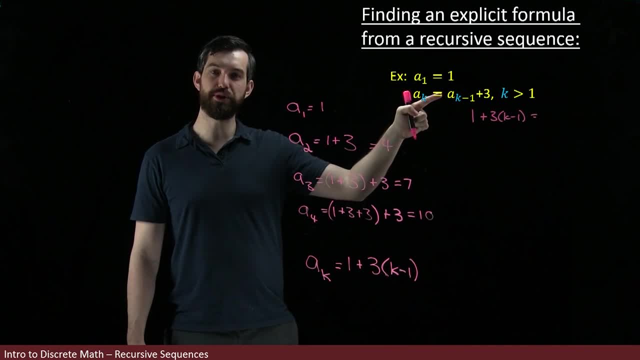 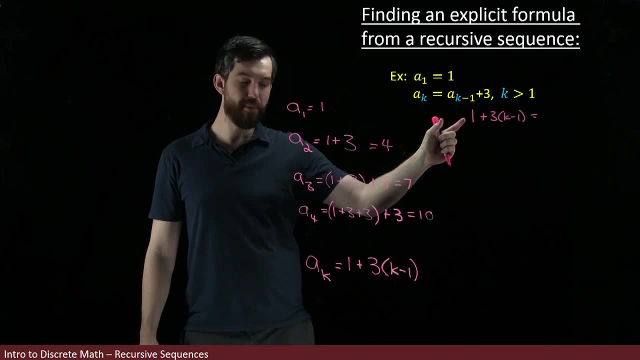 and then the question is: is this going to be equal to a if I plug in k minus 1 to it? So let's be careful here. If I want to look at a k minus 1, what I do is this is my generic formula for k. 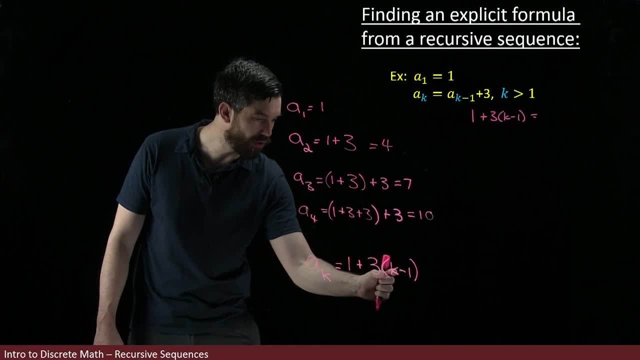 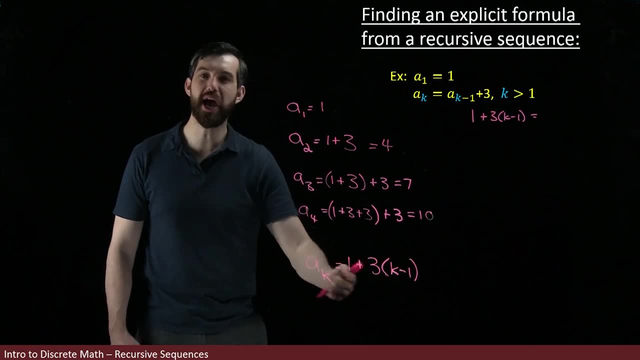 but I plug in k minus 1 here on the left and I also plug in k minus 1 here on the right, And if I'm plugging k minus 1 here on the right, then this term is going to become k minus 2.. 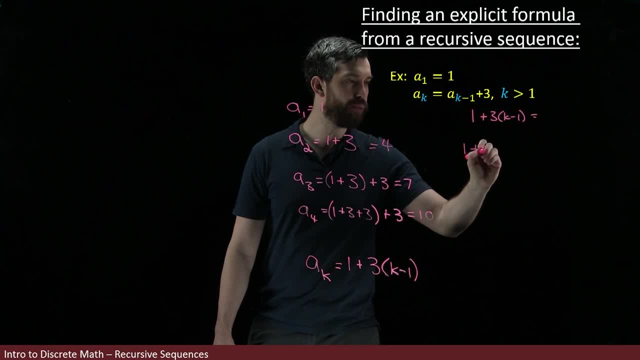 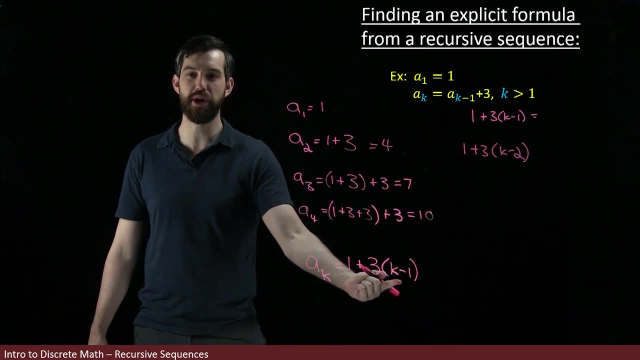 So the question is: is this equal to 1 plus 3,? and then I'm going to write it as k minus 2.. And the minus 2 comes from plugging a k minus 1 into this formula. I get the 1 more minus 1,. 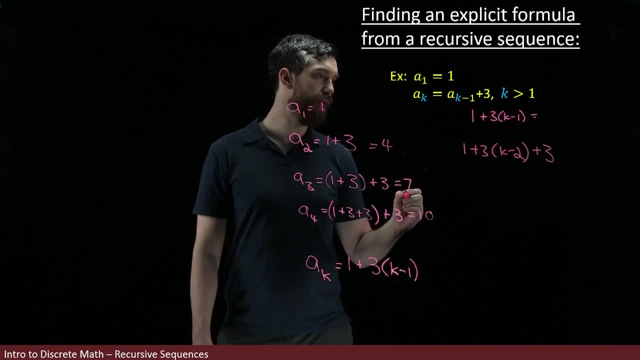 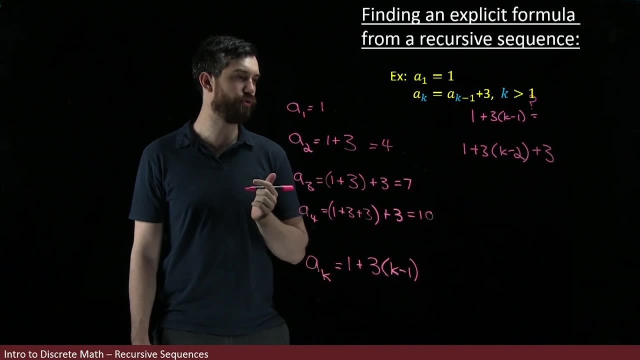 and then finally, plus a value of 3.. And this is my question mark: Is it true that this is the case? I'm trying to verify that this recurrence relation is indeed true, and I think so because I can take this formula here. 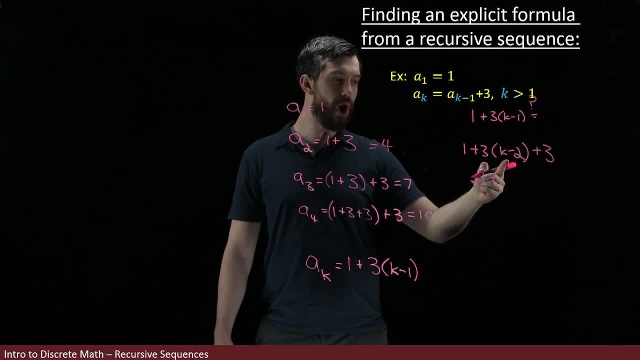 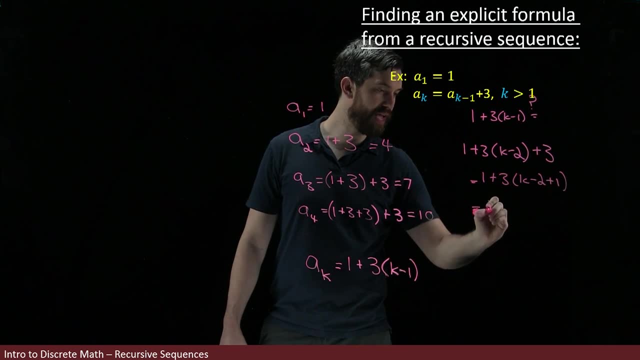 and I can manipulate it. I can say that this 3 can be brought in over here, so it's 3 k minus 2 plus 1, which is precisely the same thing as 1 plus 3, k minus 1.. And so what have I done? 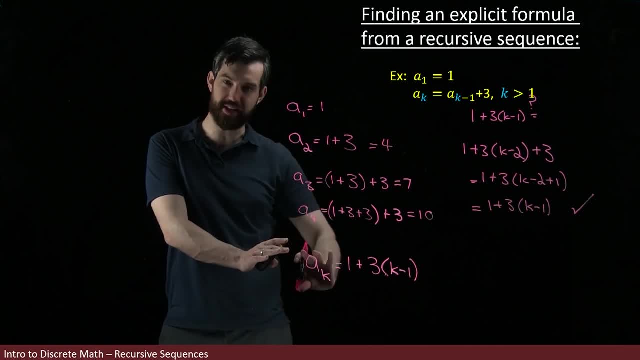 I have verified that this equation is true and therefore verified that this explicit formula does indeed match this recursive formula.